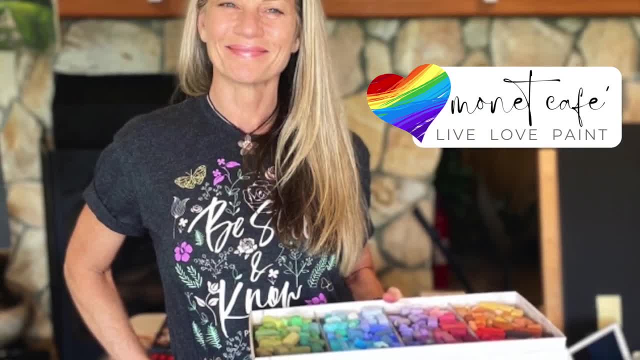 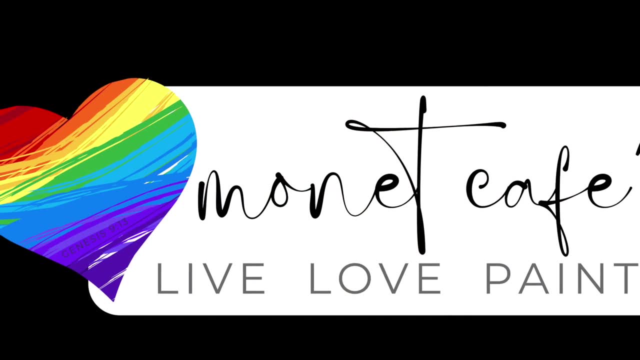 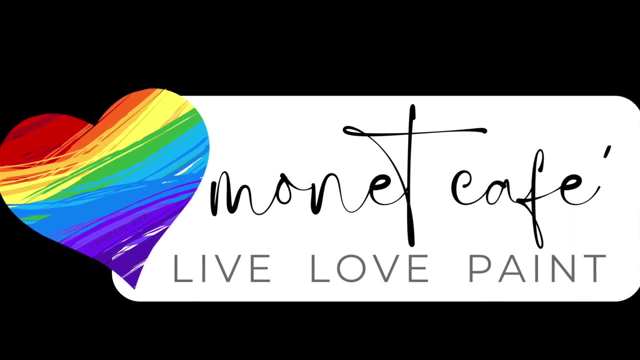 Welcome to Monet Cafe. I'm artist Susan Jenkins and I have some exciting news for all of my subscribers all over the world. Here we go. Hello, artistic friends. I want to share something exciting about Monet Cafe and its availability to people all over the world. I say that all the time. 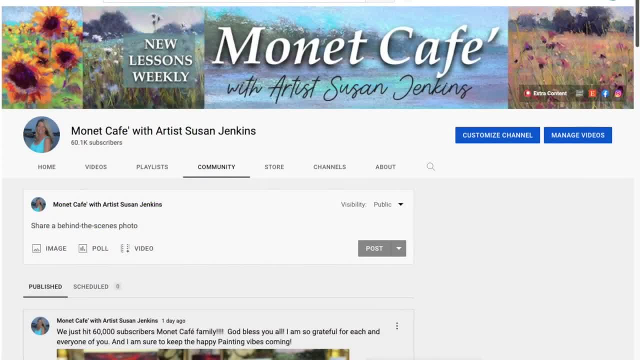 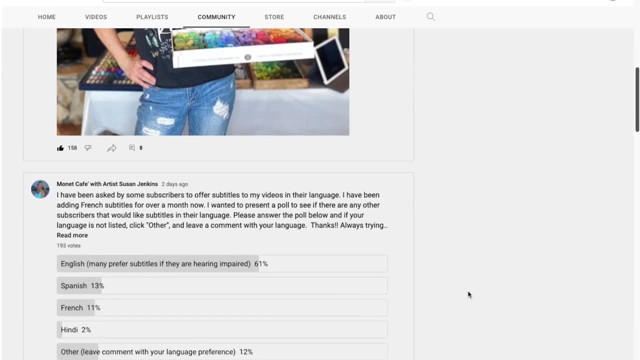 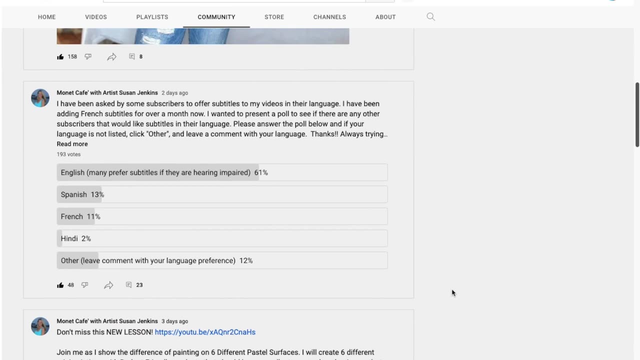 but I recently offered a poll in my community section of my channel about different people who speak different languages and I've had some requests from some in my Patreon group on my Patreon page to provide the closed captions for my French-speaking patrons and friends and I realized there were a lot of other people with other languages who may want the same. 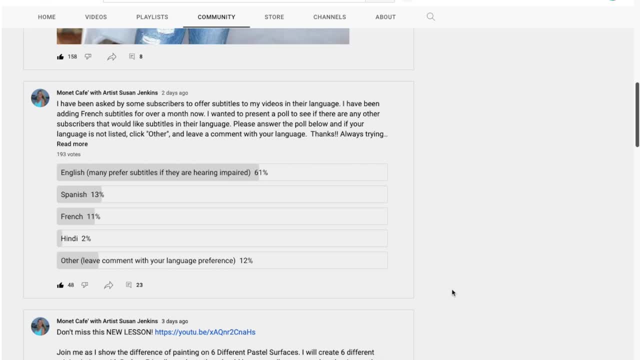 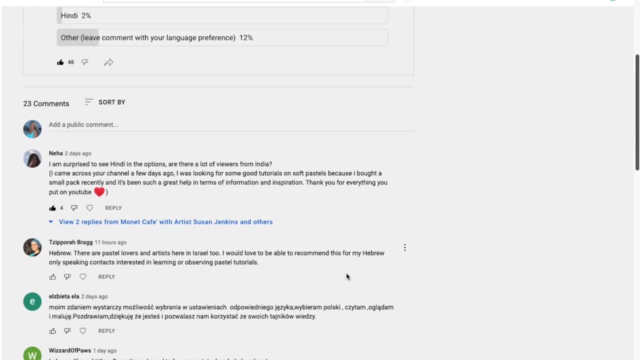 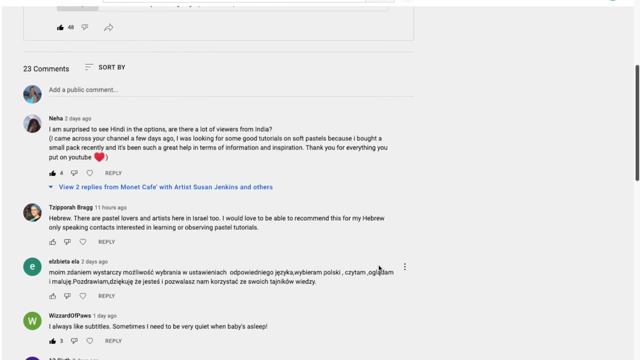 It's a little bit of work for me to do that with every video, especially if I'm translating them or providing the closed captions for multiple languages, but in the poll I was so thankful that someone answered and gave me a fix for all of you, all over the world, to have closed captions in whatever language that you speak. so that was. 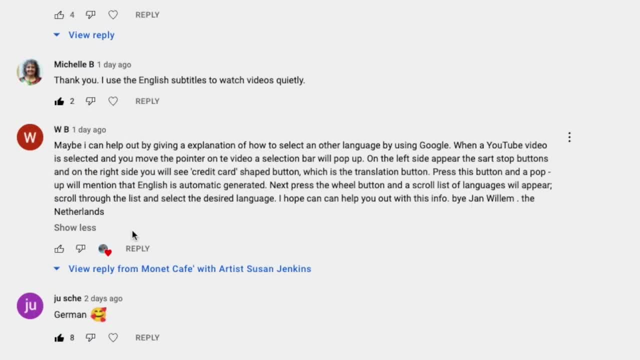 really great, and this is a comment from Jan from the Netherlands. Thank you, Jan, so much. Jan provided a thorough explanation of how you can get closed caption in any language from any of my videos, So I'm going to take you over to my YouTube page with one of my videos and show you exactly how to do that. 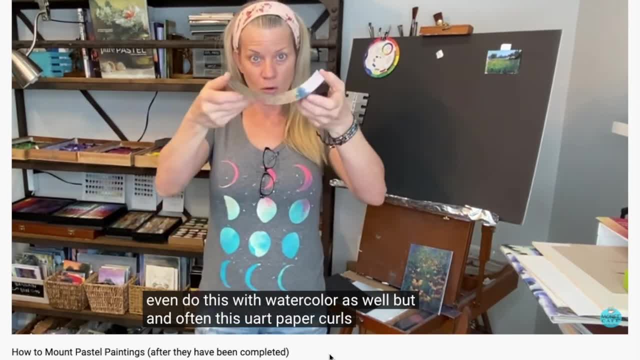 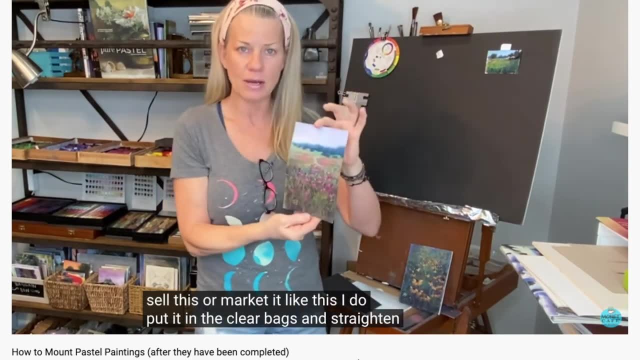 So here's a video of mine where you can obviously see me talking. I've turned the sound off so it doesn't interfere with what I'm describing here, and you can see the auto-generated subtitles below. Now. that is because I turned them on. 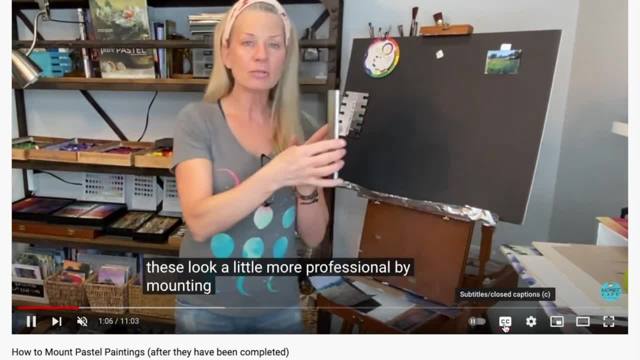 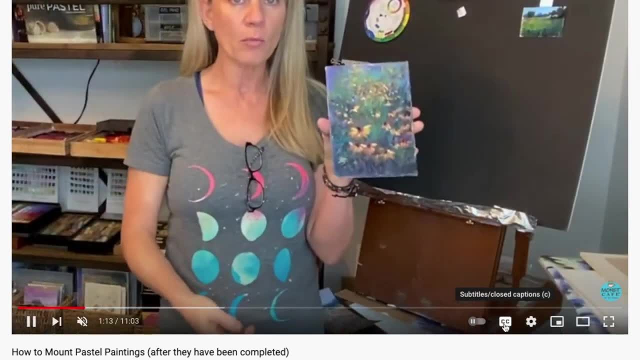 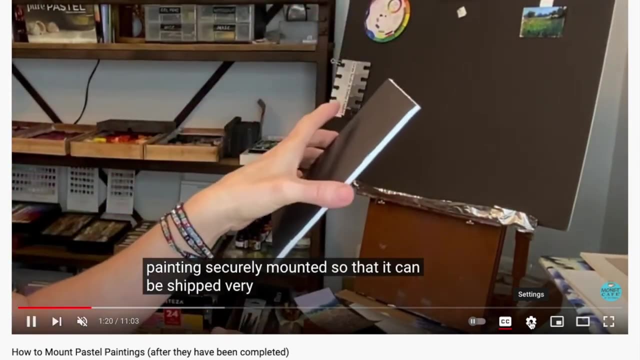 Here is the CC button at the bottom means closed captions. If I turn them off, you won't see them. Now you don't need the English subtitles, You want them in your language. So turn the subtitles on. Go over to this little gear icon right next to it for settings. You're going to click that.